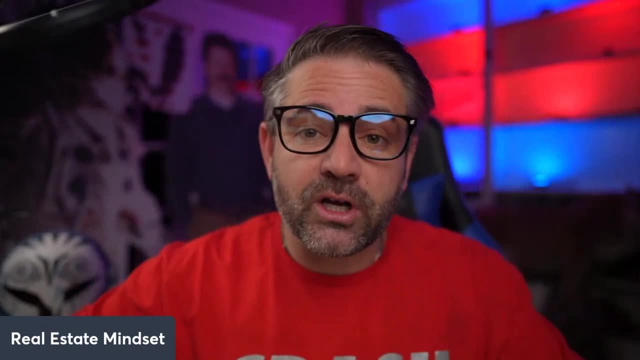 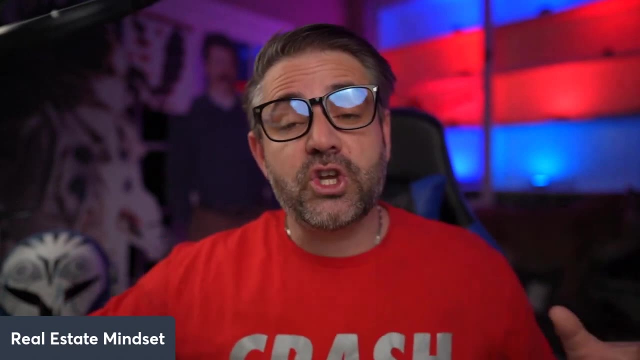 is absolutely skyrocketing as well, And so today we're going to go into a wealth of data, We're going to go into the housing market update as well as other things like demand, just to gauge where we're at in the housing market this week, And it's going to be interesting to see what the elevated 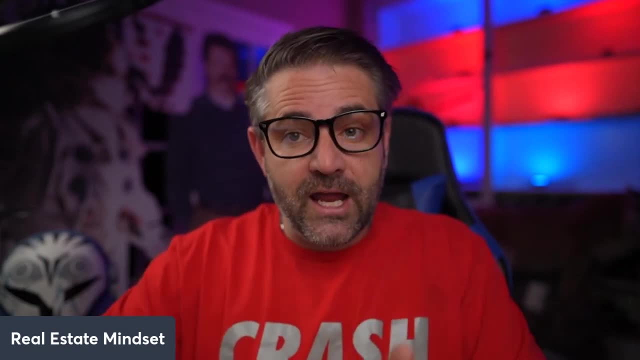 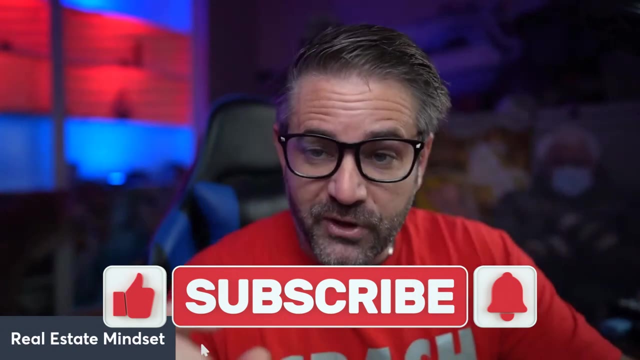 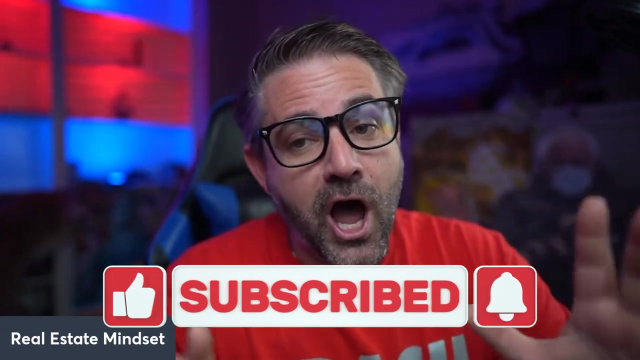 interest rates are going to start showing in the trends now that everything is greatly elevated. And do me a favor, if you guys can: if you learn something, hit like on the video, subscribe, shoot me a comment below. And also, if you have any intel and any insights, comment below A lot. 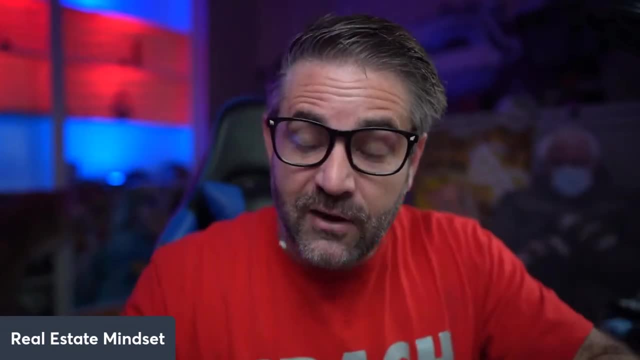 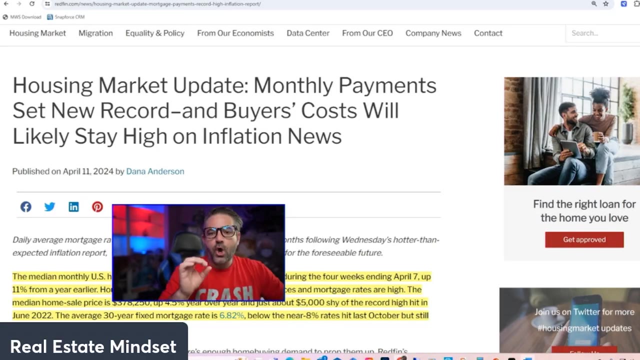 of people read those comments. Don't forget to share your Metro area. But again, if you learn something hit like Other than that, shoot me a bonkers below. Now. the name of this week's Redfin housing market update is: monthly payments set new record and. 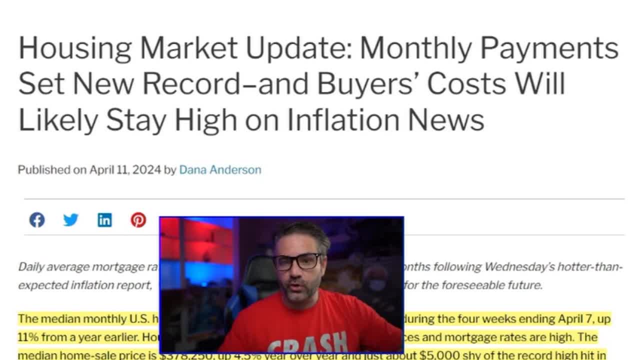 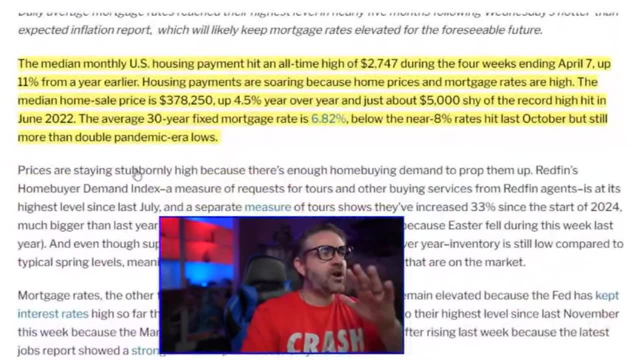 buyers cost will likely stay high on inflation news. And you guys, we have some absolutely insane trends going on right now. I mean, wait until you start reading this. I mean, not only are housing payments on an all-time record, median sales price is about to hit a. 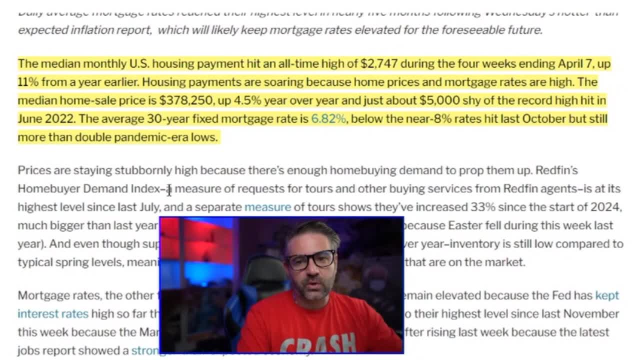 new record too, because we're going to be seeing a lot of new trends. And we're going to be seeing new trends. We haven't hit a new record since 2022.. FYI, a lot of people have said, including Dave. 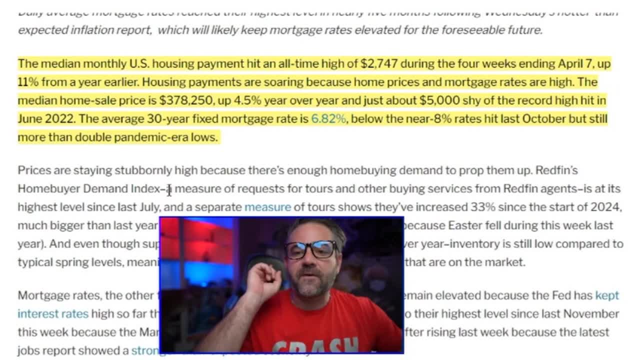 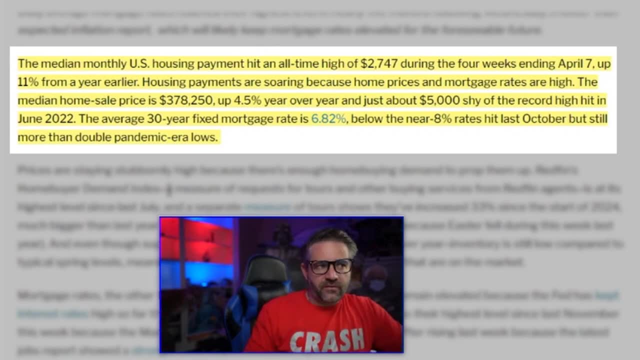 Ramsey that we have a new record with median sales price. That is false. But let's read the first paragraph. The median monthly US housing payment hit an all-time high of $2,747 during the four weeks ending April 7th. Now that is up 11% from a year earlier. Housing payments are soaring. 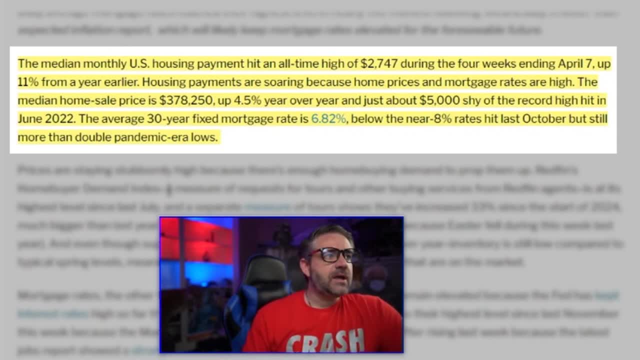 because home prices and mortgage rates are high. The median monthly US housing payment hit an all-time high. The median home sales price is $378,250.. That is up 4.5% year over year. And listen to this. This is just shy about $5,000 from the record high that was hit during June 2022.. That's crazy. 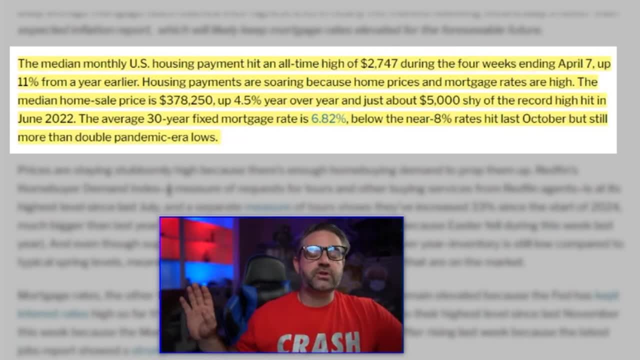 That's why I say people are spending to the end. And also this could be that higher priced houses are the only ones that are being listed because there is no affordable housing, So it could be a combo. The average 30-year fixed rate according to this article is 6.82% Below the near 8% hit. 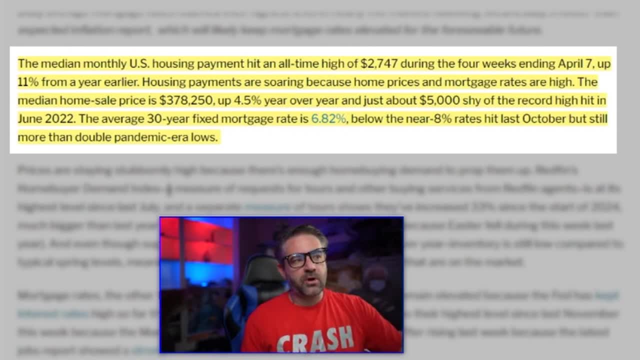 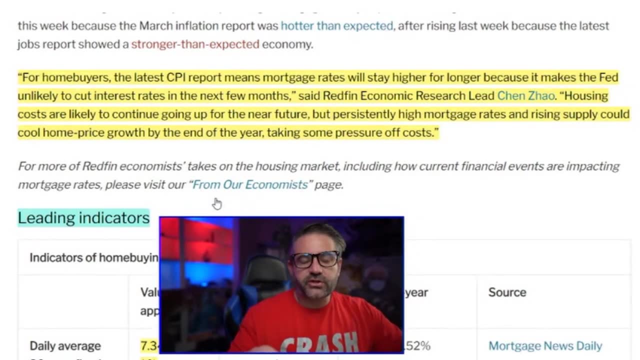 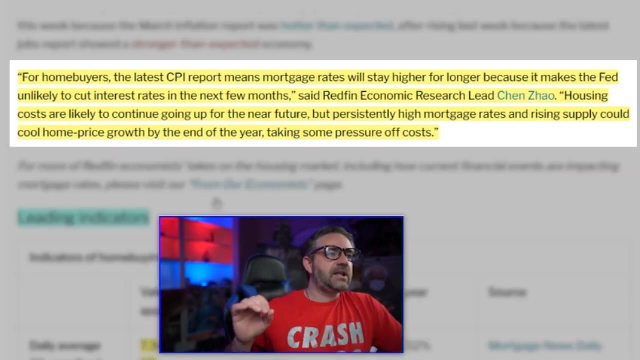 in October, But still more than double pandemic era lows. All right, Now let's read their last little, generally optimistic little paragraph from their agents that are in the field. So this is your boots on the ground. little paragraph statement here. For homebuyers, the latest CPI report means: 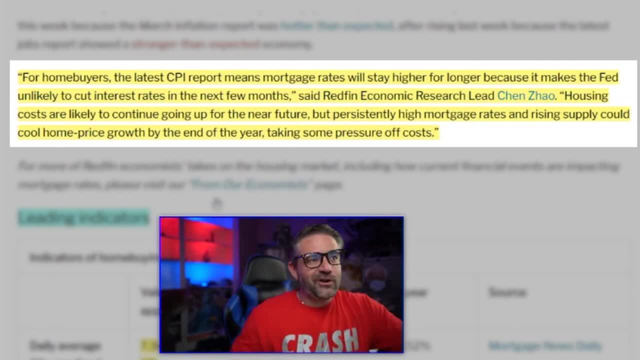 mortgage rates will stay higher for longer. I wonder, have we heard that before? I mean, is this a big surprise? Have you guys ever heard the term higher for longer? Or is this the first time you've watched this channel? I mean seriously. 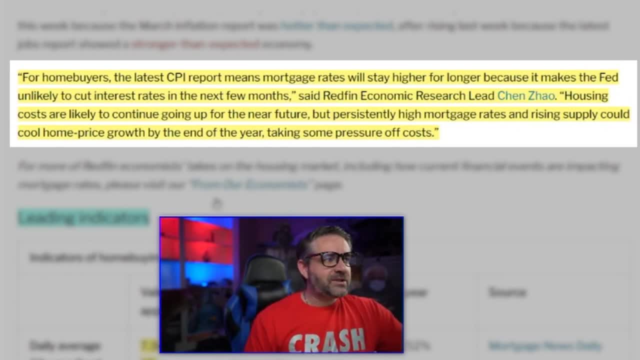 why are they anyways? Okay, Higher for longer? because it makes the Fed unlikely to cut interest rates in the next few months. Housing costs are likely to continue going down for the near future, but persistently high mortgage rates and rising supply could cool home price growth. 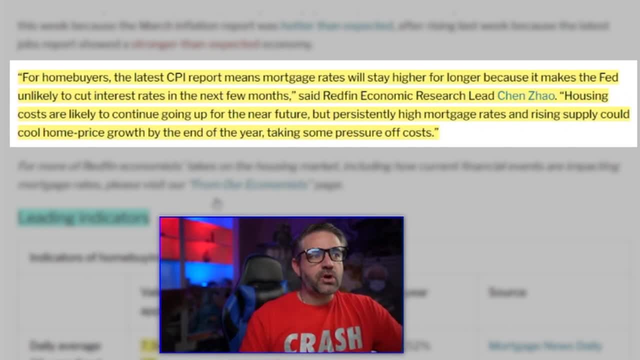 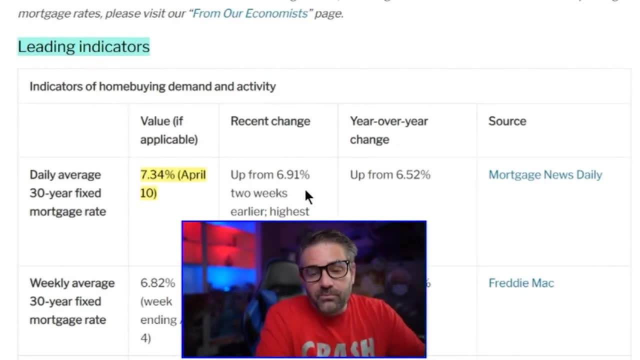 by the end of the year, Taking some pressures off costs. Hmm, Interesting. I mean Redfin is going to be optimistic. you know, do your thing, Redfin. Thank you for the data And obviously, guys, this is not the full picture. 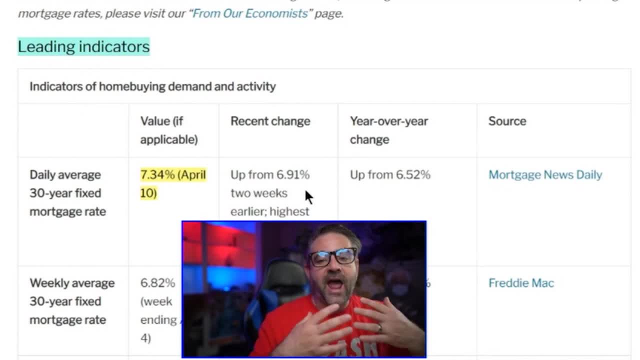 What we really need is the public, in my opinion anyways- to have access to the MLS. If the public had access to the MLS, I could train them how to be beast mode buyers- also sellers, but primarily buyers. We need people to understand how to use the data, not the emotions, Regardless. 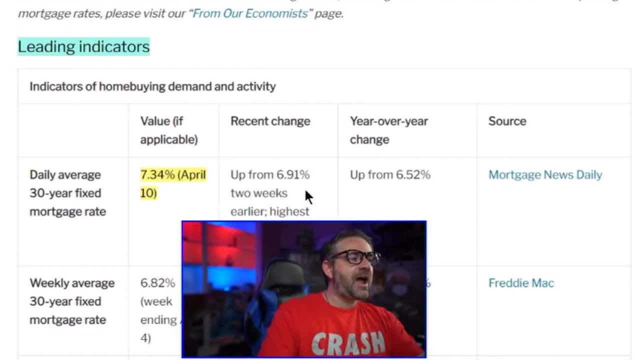 the leading indicator, Starting with interest rates. Now they have the daily interest rate sitting at 7.34%. That's up from 6.52% year over year. So right now, interest rates are are W a higher, Higher. This is the type of restriction we needed during 2023, but remember. 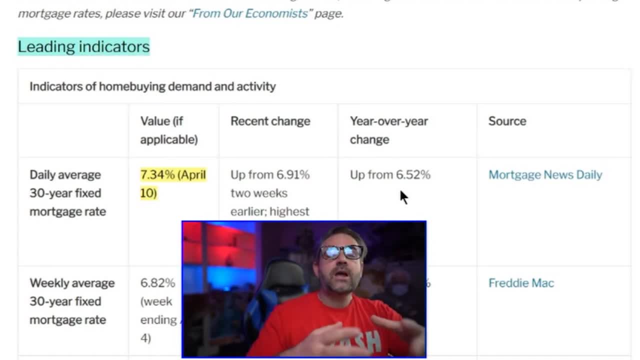 think back in time, this time last year the bank term funding program was introduced, basically about a month prior, and that basically allowed liquidity in the banking sector As those bank runs started started. You guys remember the bank runs last time we had. you guys remember that similar to 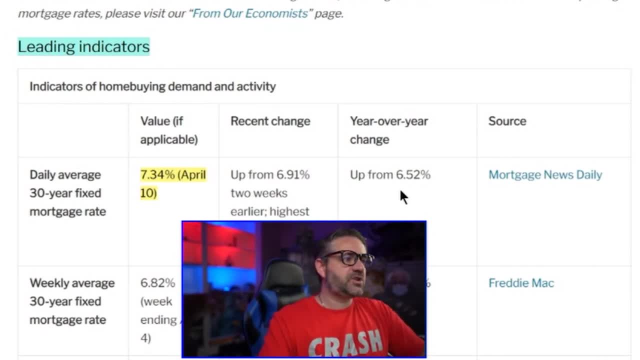 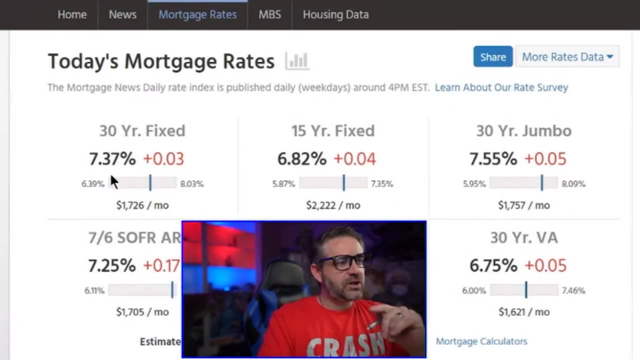 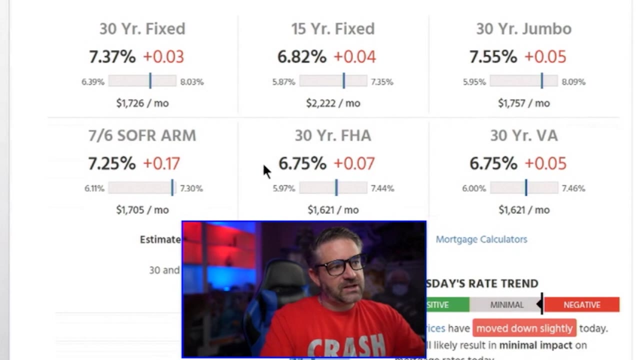 the great depression bank runs right. Very interesting stuff, But, regardless, you guys were sitting at 7.34%. Now, from the date of the recording of this video, interest rates are sitting at actually 7.37%. I want you guys to also take note here that FHA- FHA is sitting at. 6.75%. That is lower than 15 year conventional mortgages. Isn't that surprising to you guys? Also, I want you to remember: generally you can get a better deal shopping a broker versus a direct lender. Now, when we look at things like demand, starting with mortgage, 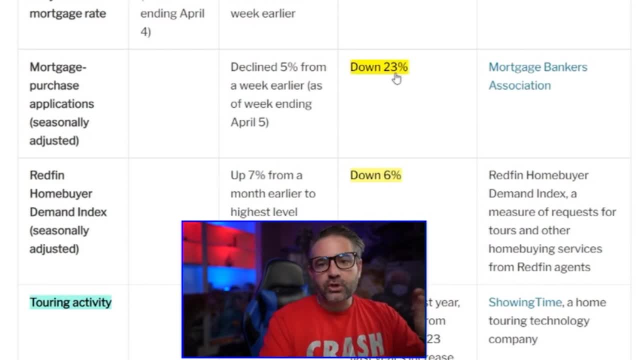 purchase applications. this is down a whopping 23% year over year And we were already at his- like 1990- lows. So we're starting off 2024, even though it's spent to the end, at least we're starting off with sales in the gutter and getting even worse than last year. 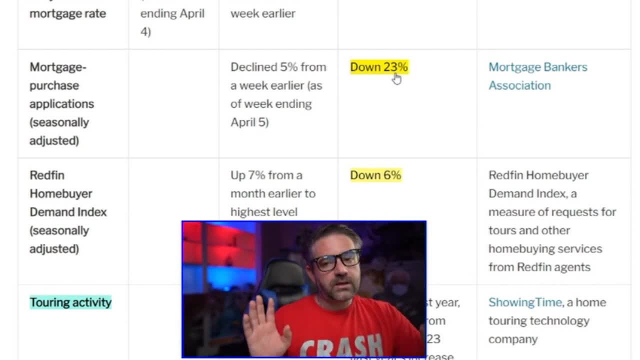 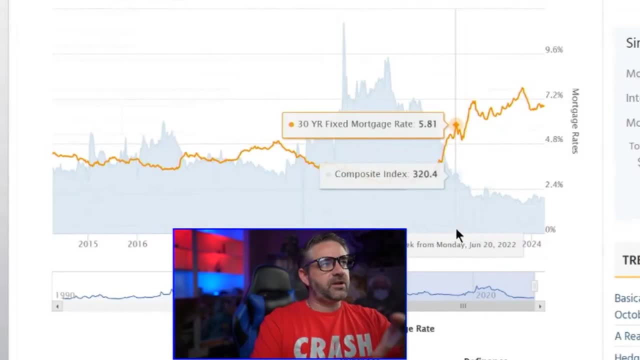 And 23% is substantial again, being how bad it was last year. Now it's also saying Redfin home buying demand is down 6% year over year as well. Take a look at this data from mortgage news daily. This is really painting the picture of how low mortgage purchase applications are right now. 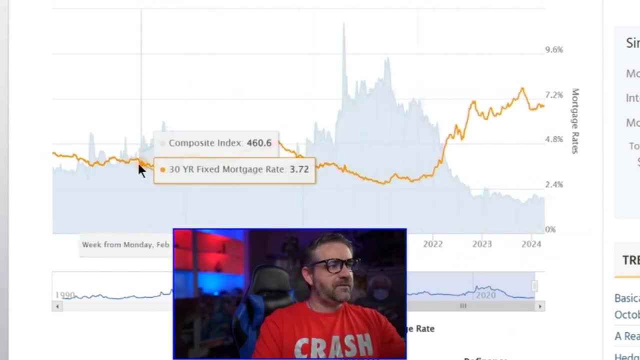 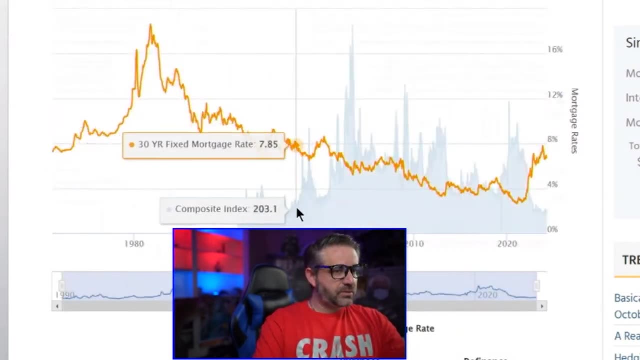 The index is about one 95. The last time we had one 95. I mean, we haven't. I have to actually max this chart out and go all the way back to geez. you guys, I'm going to look at this. 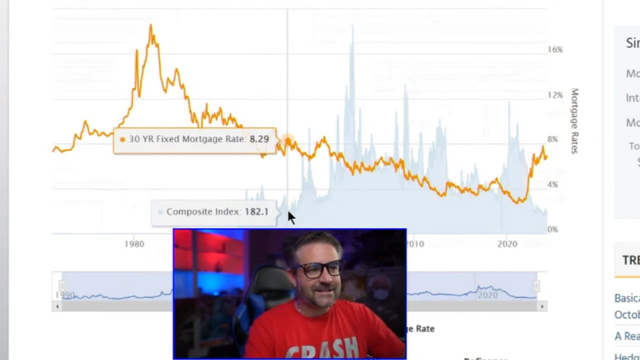 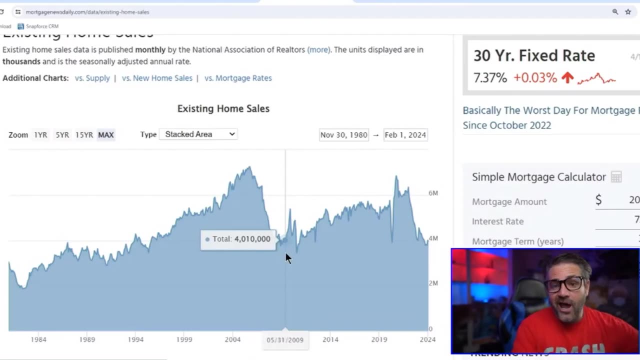 I mean, what is this? January 24th 1996, and it's getting worse. So demand absolutely in the gutter right now. Now we also see that when looking at existing home sales- So to the bulls you can't say the housing market is strong- We know that we need more affordable housing. Yes, We also know 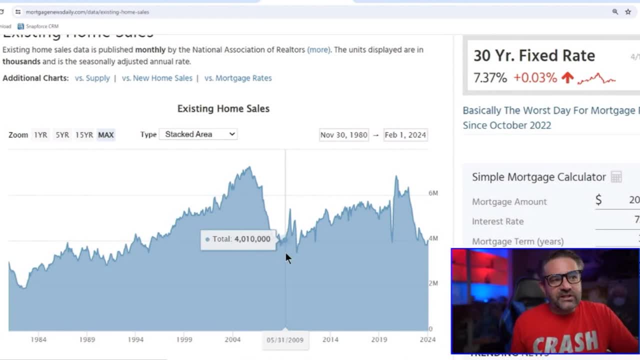 that there's 15 million vacant homes. We know all of these things, but regardless, a lot of people aren't buying. There's still a lot of people buying. That's not good. But look at this, guys. We're sitting at right now, 3.9 million. Okay, So we're under 4 million. Last time we were under. 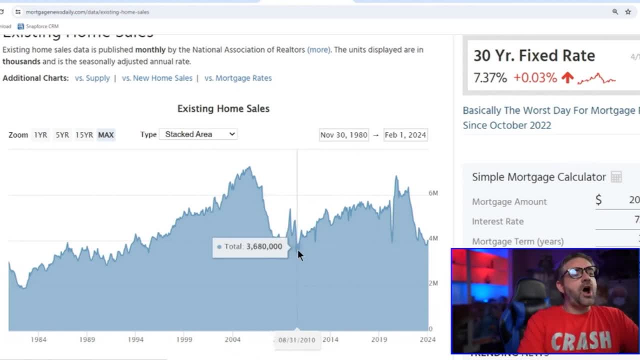 4 million was during the GFC, right about here in August of 2010.. Now, prior to that, we had to go back again to the 1990s. So the fact that interest rates have remained elevated going into spring is a great thing for the housing market, And so long as we can stay elevated in the situation this is. 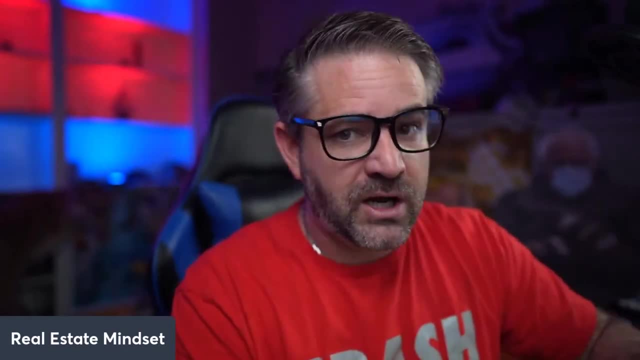 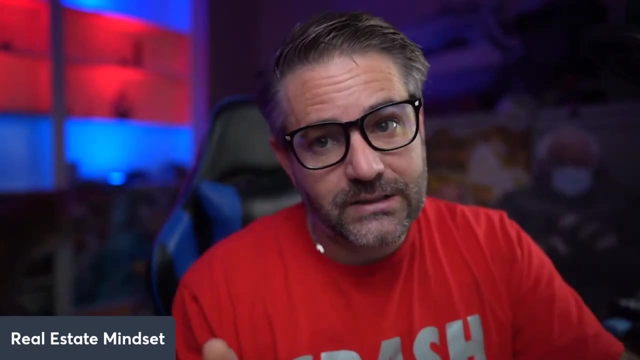 what we want. Now I'm going to tell you guys what we don't want. We don't want some black swan to come in and the feds have to cut interest rates before we have a proper reset and rather- and I hate to say this- unemployment, If they lower rates before unemployment or before some type. 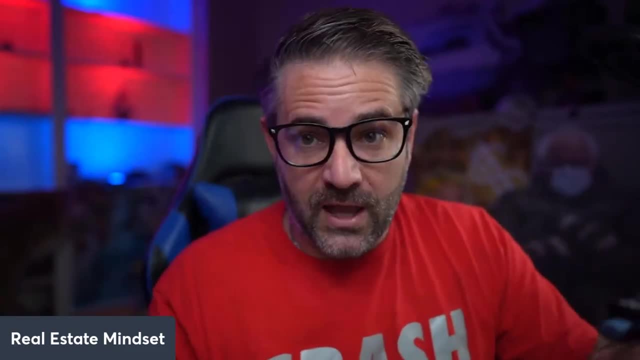 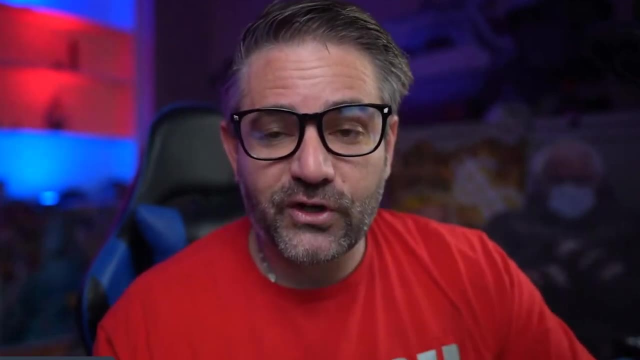 of event happens it may. all of this may be for nothing, but even so okay. even if this was all for nothing, 90% of America still can't afford the house and therefore things are still not sustainable. Anyways, 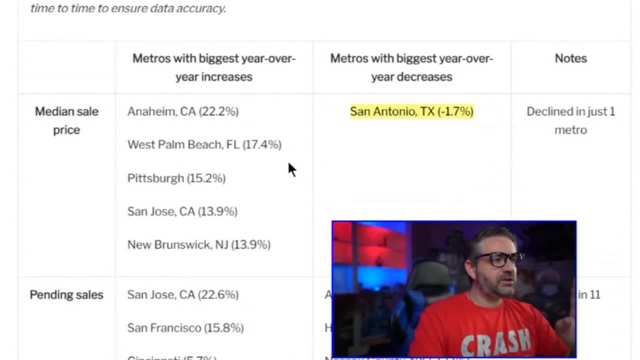 let's go back into the info. All right, y'all. So take a look at this week's winners and losers. Number one: Anaheim. usual suspect, Anaheim, Now Anaheim, sitting at an increased year over year of 22%, followed by West Palm beach, Another usual suspect- massive year over year. quote unquote. 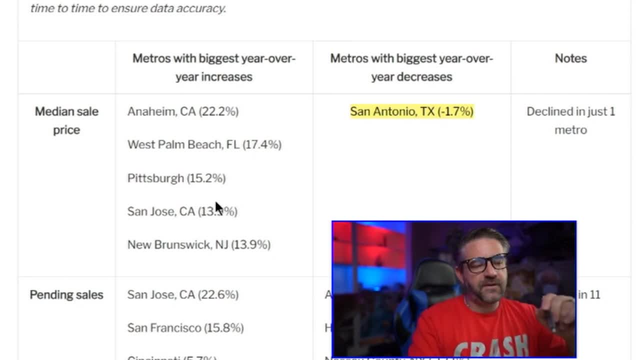 growth right there at 17.4%, Pittsburgh at 15%, San Jose at 13.9, new Brunswick at 13.9 as well, with only one Metro area, which is San Antonio, Sitting on the year over year price decline list. I mean, Texas is always in the. I mean 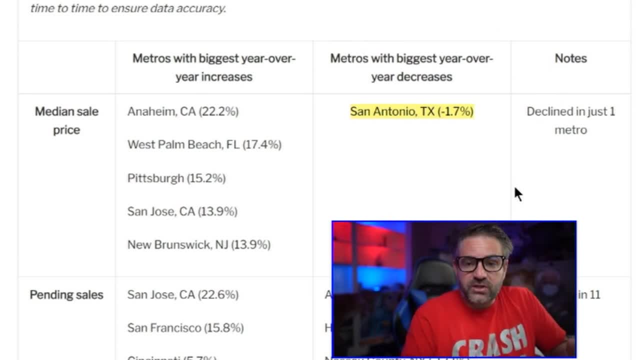 do you guys see why it's for me being in Texas, Houston, Texas- this is so easy for me to see. but regardless, you guys, San Antonio is down 1.7% year over year. I also want to bring this up. 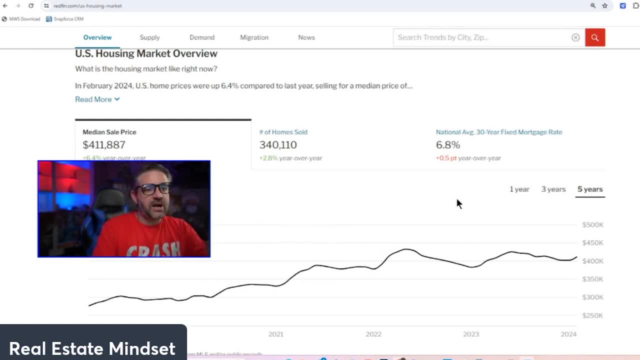 The fact that we didn't hit a new peak in median sales price last year. Okay, A lot of people like: Oh, the housing market rebounded, We're all good. Yes, there was a rebound. I think it was more of a. 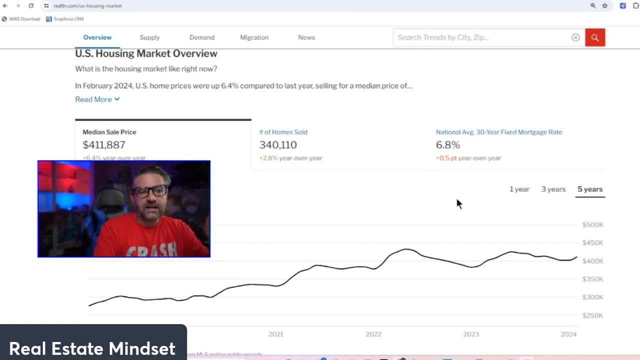 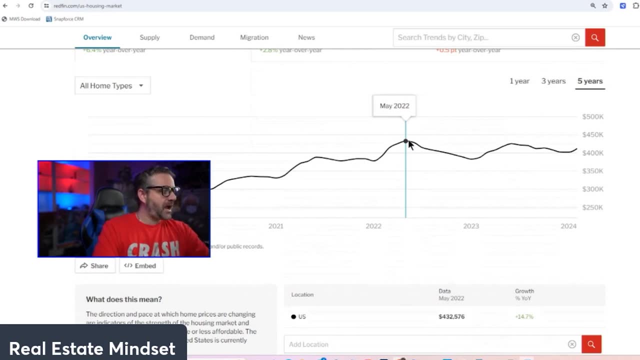 dead cat bounce and it was a beast, but we still didn't hit. Hit a new record. The record was essentially in may of 2022. We were sitting at 400 right here: 432,576.. Okay, That was in 2022. Now we peaked out in 2023 at 425,000.. That was June of 2023. 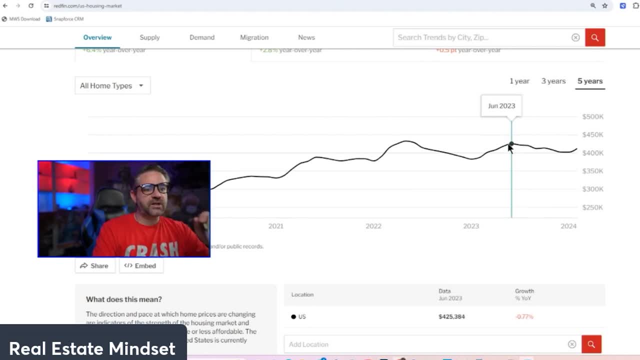 And for the remaining part of that year you can see. prior to that, actually, it was on the year over year decline list. Do you all see that? So we started 2023 with homes down year over year. Okay, You all see that. But again what I'm saying: is, we did not hit a new peak. So not only our transactions in the gutter, we still didn't hit a new peak. Okay, So you can still argue that there's still no equity growth because it takes money to sell your house- roughly 8%. right, We get that. as America, We know that. 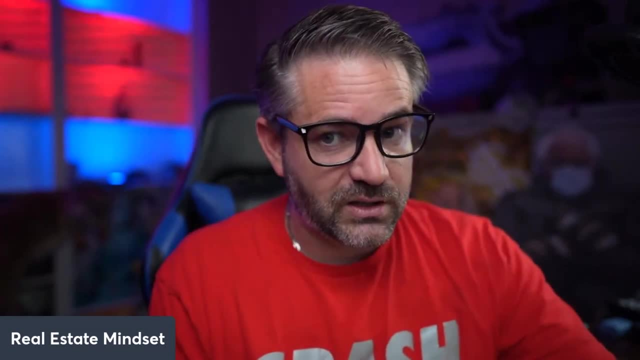 right, We get that by now. It costs money to sell your house. I mean, there's lawsuits about this. Everyone knows this by now. Come up below. please Give me a bonkers as well, If you haven't already. 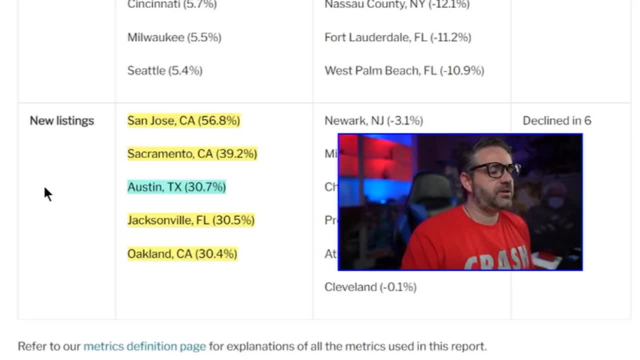 but come up below. Okay, What are your thoughts on all this so far? Now, before I get into the charts, take a look at this, guys. This is what I'm talking about. This is what I'm talking about. This is new listings. Now we want to keep our eye on new listings because we need inventory In. 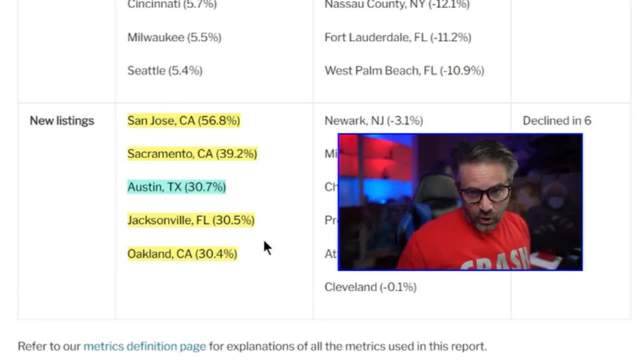 fact I've been saying we need 900 to a million active units sustained right, So for a period of time for prices to start going down again- at least that's my hypothesis based on the last three years- and the price declined during that time. Now take a look at the new listings. This: 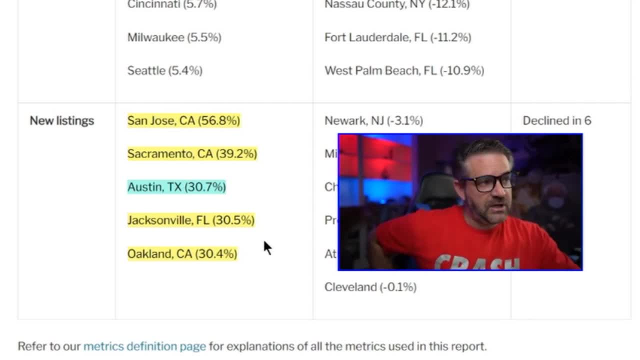 is insane. Although San Jose is blowing up, apparently, in median sales price, it's the new listings are freaking, exploding guys: 56.8% year over year. Wow, Okay, That's, that's a. so we should start seeing prices like flatten out or at least go down in San Jose, Right Look. 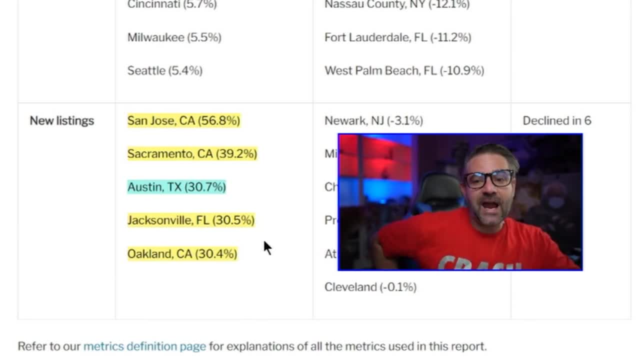 look at the inventory now. Sacramento's also on that list at 39%. Austin, You guys, Austin is going to be back on the year over year price decline list. The new listing surge in Austin: 30.7%, followed by Jacksonville, Florida at 30.5% and Oakland, California. 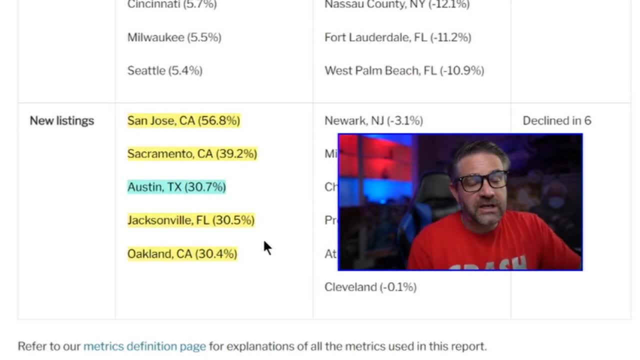 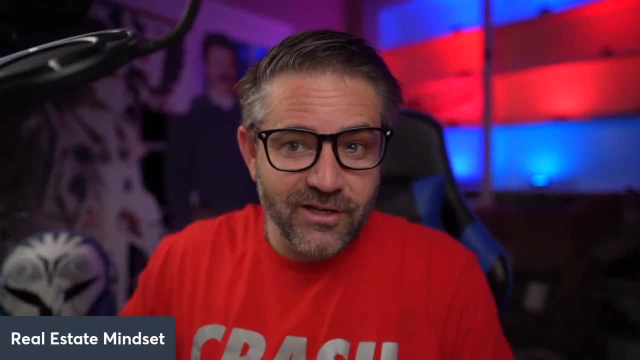 California at 30.4.. Keep your eyes on Austin and San Jose. I mean seriously, guys, is this data not absolutely wild? Y'all see what I'm saying: Spend to the end And yes, yes, I am talking to. 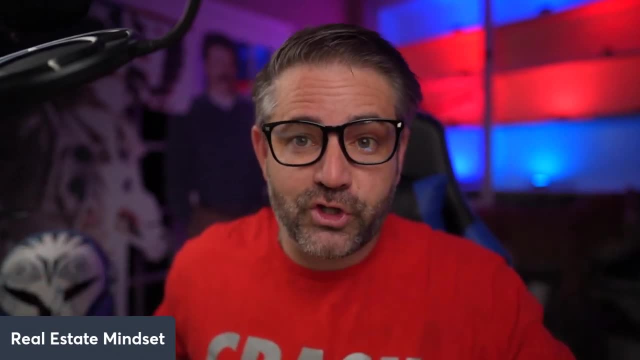 you, 20 year old Travis that lost everything during the GFC spend to the end. That's exactly what you did. It hurt. It hurt to say that, hurt to say that. let's move on to data visualization. All right guys. So, starting with median sales price, this is, this is bananas. 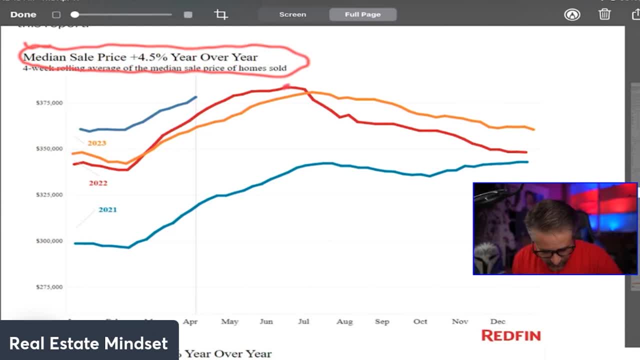 Now, remember you guys, we still didn't hit this record here. Okay, So this is the record. Okay, This record was from 20. 22. So, year over year over year, we still haven't hit that new record bulls. Okay. Now again, I constantly say this. Some people could still find a good deal in this. 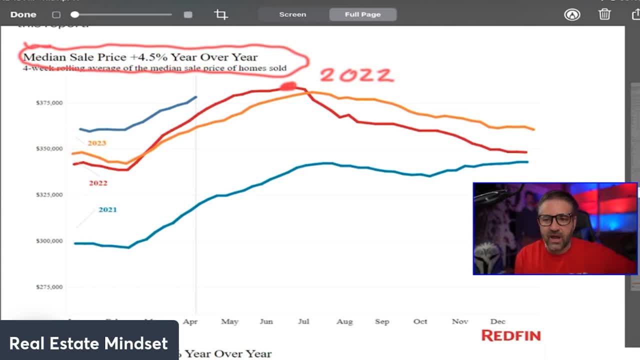 market. You gotta use data, You gotta have patients, all these things. I have a. you know we discuss this all the time on discord, but regardless, you guys look at the trajectory week over week. This trajectory is nuts. So now, again, this is demonstrating they're. 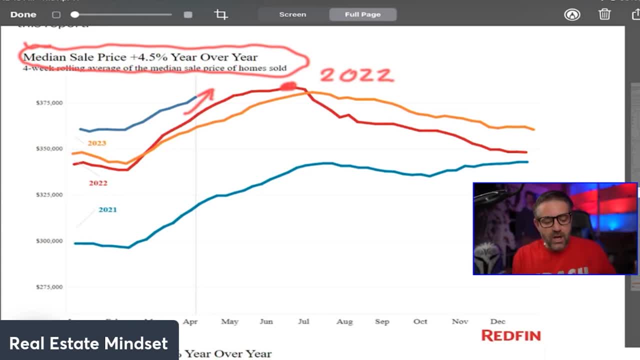 still people purchasing. but it also can be the fact that we just don't have lower end houses on the market. They get scooped up before the more expensive houses. Now I don't know that for sure. I'd have to dig in more. but regardless, this son of a gun is skyrocketing in the face of interest. 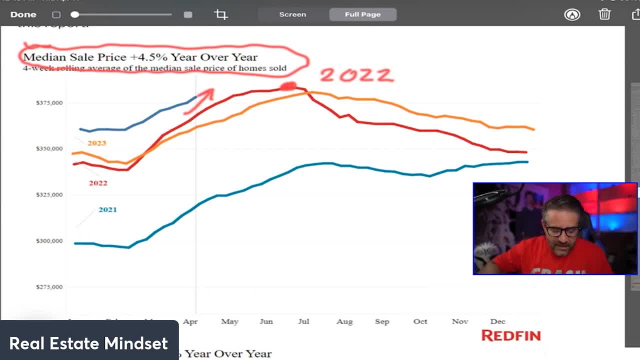 rates being in the 7% Again, And that's why I'm saying we need more active units, around 900 to a million. Now remember this: in 2022, this period that I'm circling- we had massive price decline that exceeded the GFC. Okay, During this period of time, we had roughly 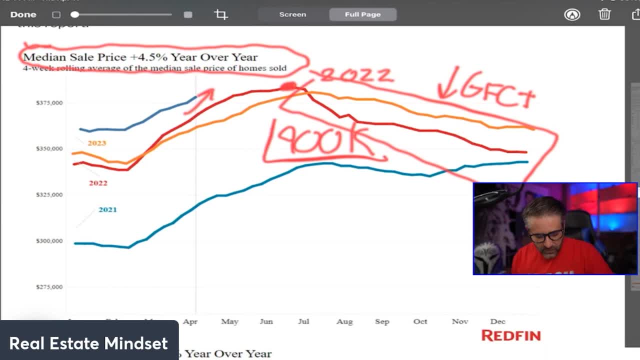 900 K active units. So that's why I'm saying it will be interesting to see if we can get to that amount again, but, unlike 2023, sustain it. Okay, That's what I'm saying. We've already seen what. 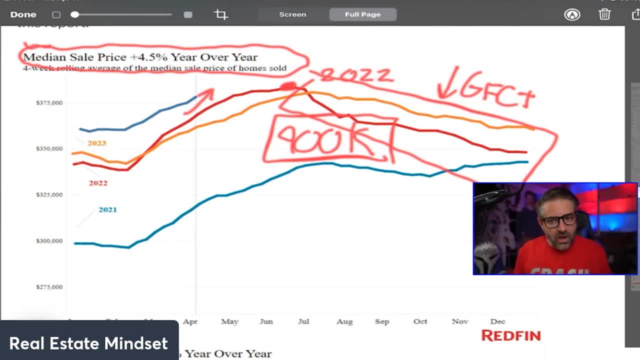 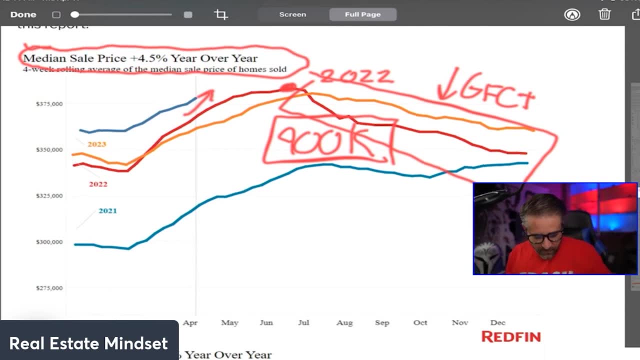 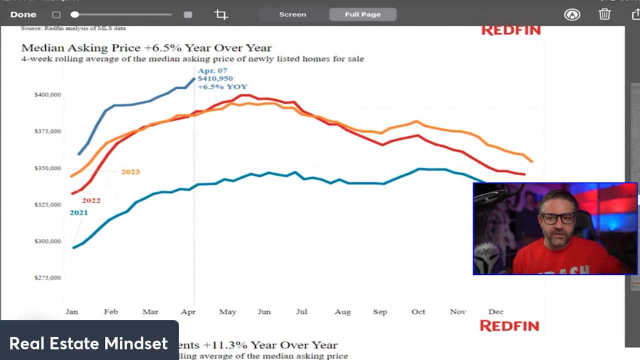 happens when we don't sustain it. The market rebounded. Obviously, I don't think that can go on and go on forever because of the unaffordability, but nevertheless, median sales price is up 4.5, and that is year over year. now here's why i think it could be less affordable houses on the market. 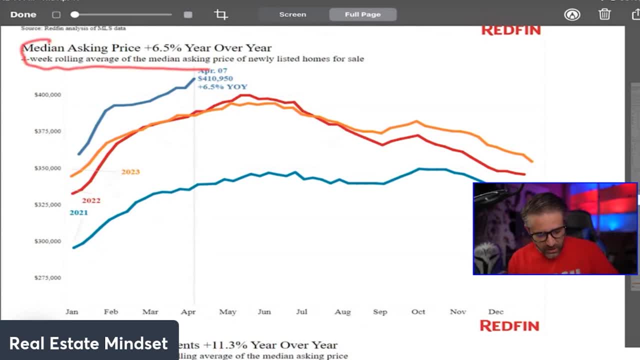 and more expensive houses on the market because median asking price has skyrocketed week over week. and remember this: data we're looking at is week over week data, but we can also compare year over year, year over year over year over year, but the trajectory of these lines is all week over. 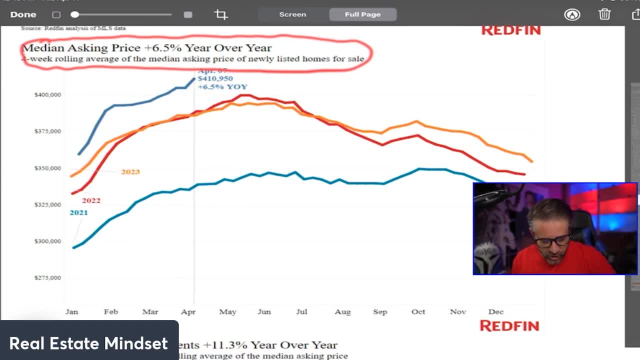 week. some people don't get that. still, it's crazy to me. but look at that trajectory and that's why i'm thinking like maybe it's it's the more expensive houses are being listed and the less affordable ones are just not being listed either way. that is an alarming trajectory and it doesn't. 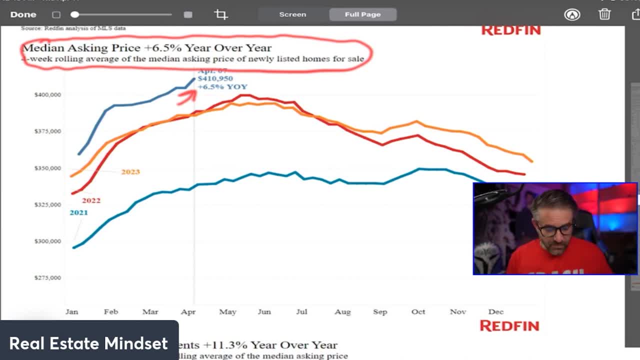 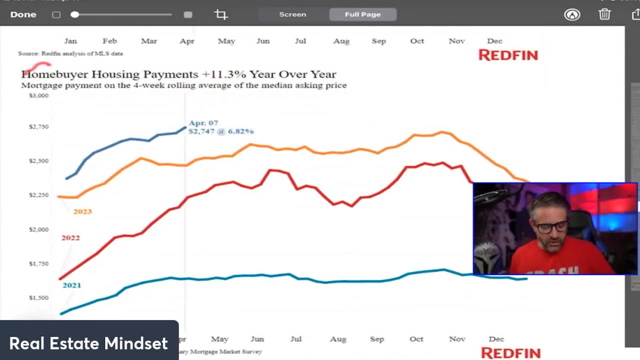 make sense and i'll show you that as we move along here. but that is up 6.5 year over year. that's insane. now take a look at this doozy. we hit a new record high, unfortunately, and actually this is fortunately. i think that the market needs this, because the market needs to calm down, even though 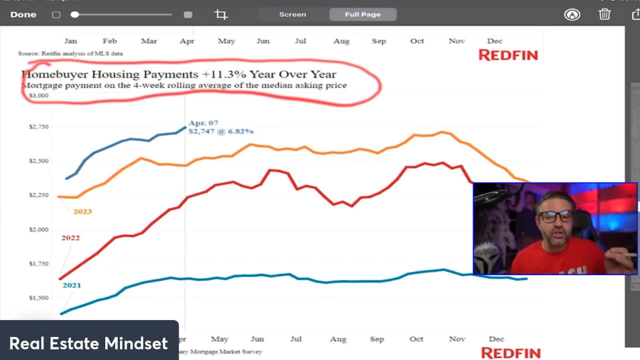 it's all the sales, everything record low. there's still again. there's still some people buying and i'm talking to those people. but home buying, housing payments, right now, year over year, which is here to here, because it was already so unaffordable last year, so unaffordable last. 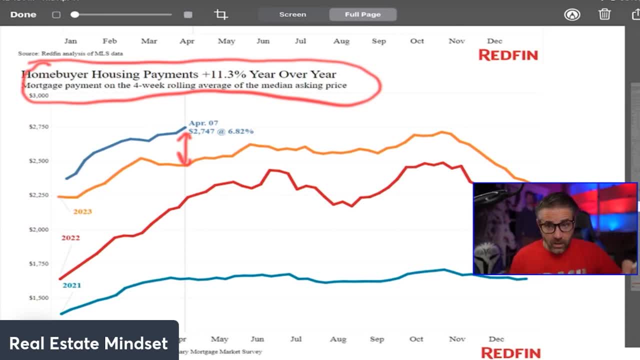 year, but year over year is even higher, even higher by 11.3 percent. we basically need home prices to go down about 60 percent. okay, i think we all- or we need to make 40 more in income or rates need to be two percent, and that's why i'm saying this whole. 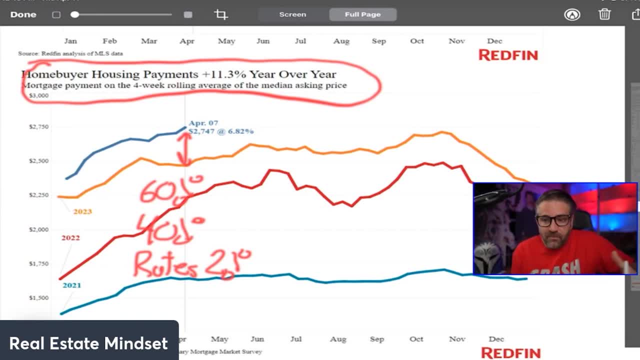 foundation is not going to last. it's built on emotion. it's not. it's built on emotion, you guys, and a lack of supply. a manipulated, really synthetic lack of supply. it was a manipulated situation, okay. it's artificial lack of supply because of the lockdown and the money printing. 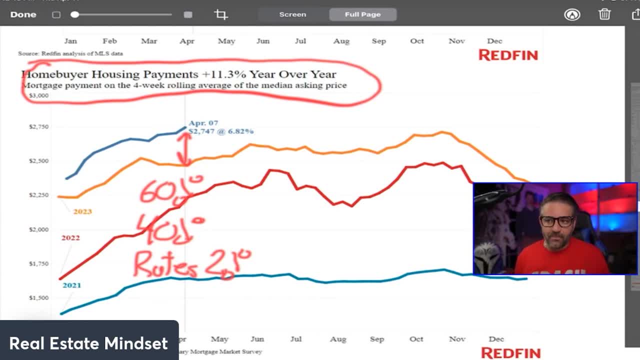 but regardless, unaffordability is king right now. and look at again when we look at three years ago. we look at three years ago. look at that, i you know from here to here. okay, that's insane, it was about sixteen hundred dollars. okay, so three years ago we're about down here about sixteen hundred dollars. 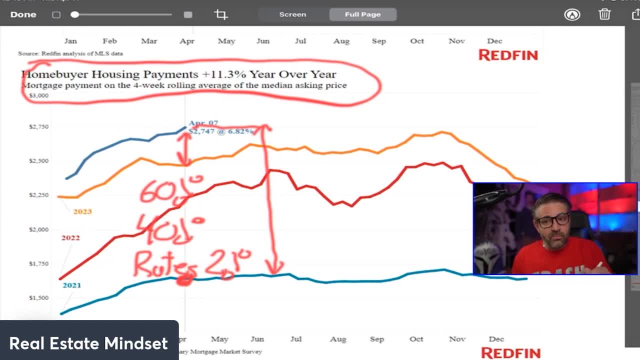 it's eleven hundred dollars more every single month. that's take-home money. that's not gross, okay, your gross income is before taxes. that's out of your net income. this is harsh. this is harsh right here. that's what i'm saying. hold up, okay. and if you are gonna buy, for the love of god, please use some fundamentals. 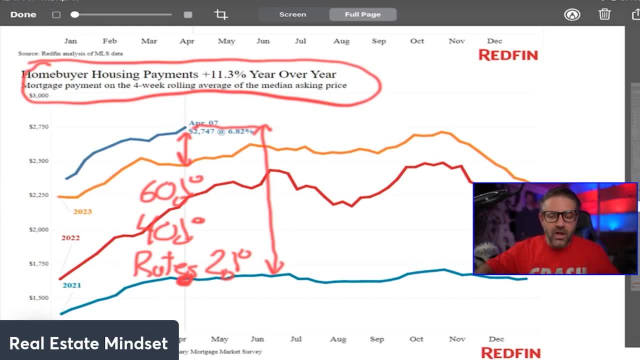 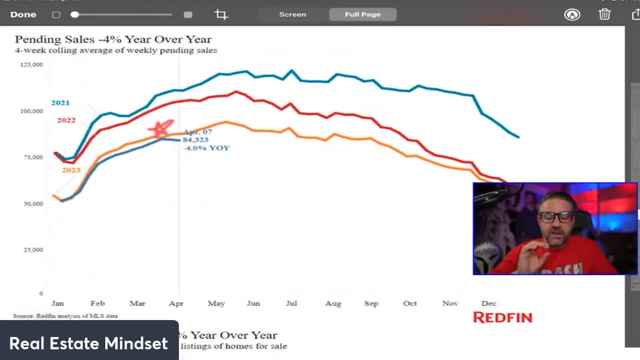 to survive through a recession that we haven't even started, although when you look at deficit spending, we've been in a recession since about 2020. i won't go there. let's move on. now. here's a data set where i think we're finally starting to see those seven percent interest rates shock the. 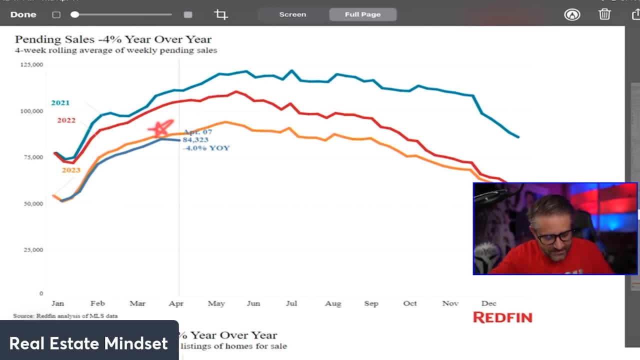 market, basically the market hitting the wall that's impending sales. okay, so again another demand matrix and look at the trajectory. look at that. it's like it hit a brick wall and is now going down. now, unlike some of the stuff that we just went over, this is absolutely great news. why? because this: 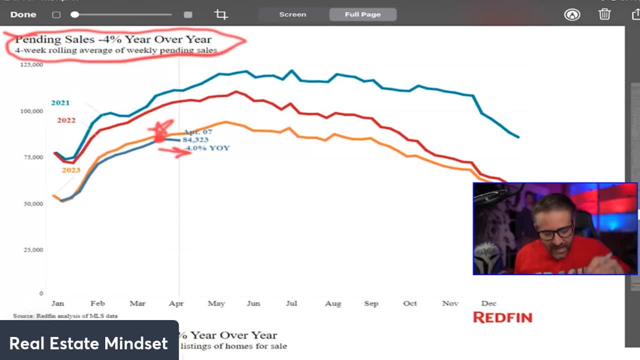 is the opposite of seasonality taking over this trend. remember, guys, we are going in and now in, spring, home buying season. so generally this time of year, pending sales go up, they don't go down, but money is shut down like a miss happens whenever we can. but one thing, though, is you know we'reрузik. 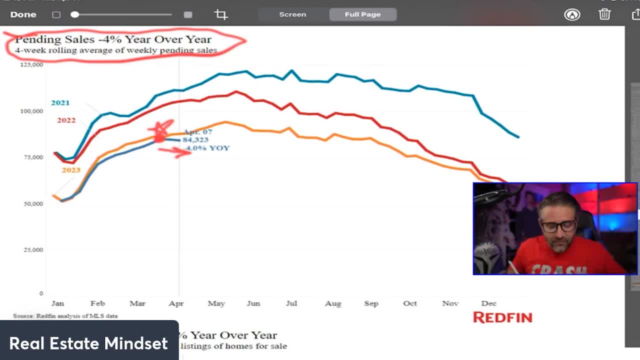 we're doing land two account families for free and that's why we're in this hard time. right now we have Tiananmen Square mead two friends who have been disqualified and invested. savings last three or four years were not even realized. so even before the dark, students arecap ahead. so what's the real moneydose here? back to before the Experts. yes, look at this chat for and the About of the comme house presentation. what are the reality of dollar back and forth and new revenue observances? what's your example of what you see here just saying: let's move on. here's new listings also vision trading. 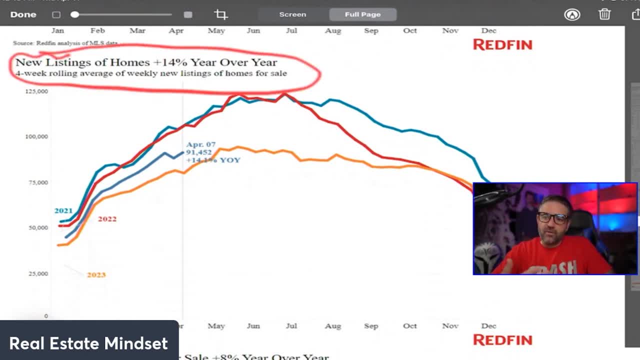 very, very good information, you guys. new listings 14 year over year. this is good. this means that it is working still slow. i know everyone's like my gosh, this is slow, everything's taking so much time. but it does take time. unfortunately, the housing market is not the stock market, so we're up 14.1. 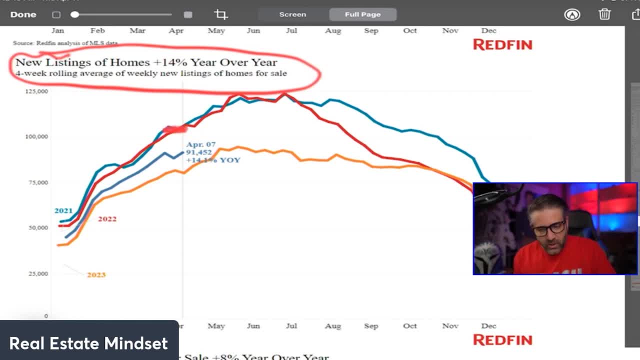 but we're still under 2022 and 2021. just wanted to make that point. we're so, we're headed in the right direction, but don't forget, there's still that golden handcuff effect. so this is great growth and meanwhile, understand, we still have that golden handcuff effect. so when those rates 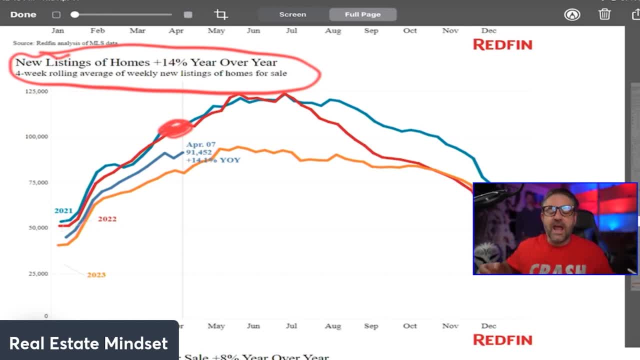 do go down. that will be met, depending on how they go down and the circumstances at which they do drop rates. depending on all that, we will have more inventory from low rates because there's a net difference, which means not everyone that sells their house buys a new ones. the last report, i 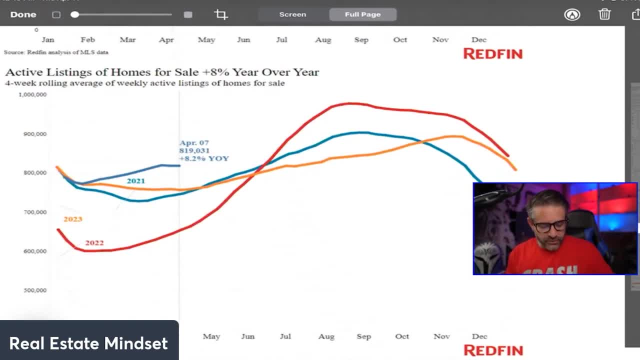 read was a 30 net difference. this is also some great news right here. this is active listings of homes for sale. we are up eight percent y'all you year over year and this is a four-year high for this time of year. so this is actually really really good news. up eight percent year over year, again sitting at 819. so we're at 819. 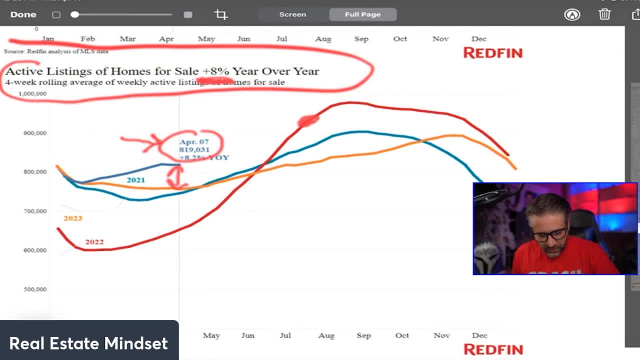 000 again. this is where i think we need to be. so we need to be right over here, because during this period- right here, okay- is when we had prices go down and go down faster than normal seasonality and faster than the gfc. before anyone starts playing the seasonality card. i've already looked. 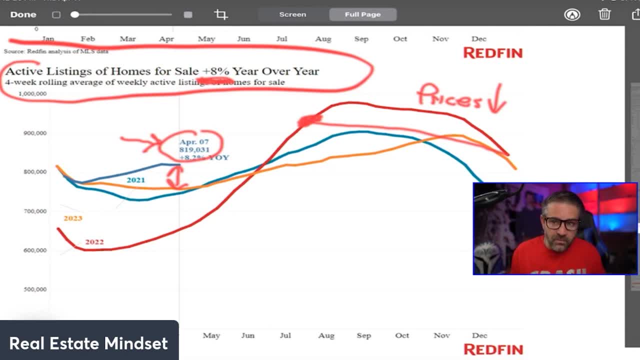 at all that info. okay, we need more inventory bottom line now. i don't like it kind of balanced out right now. what we want to see is we want to see the same thing that happened in 2022, from this time to this time, where active units skyrocketed. okay, so the fact during the last 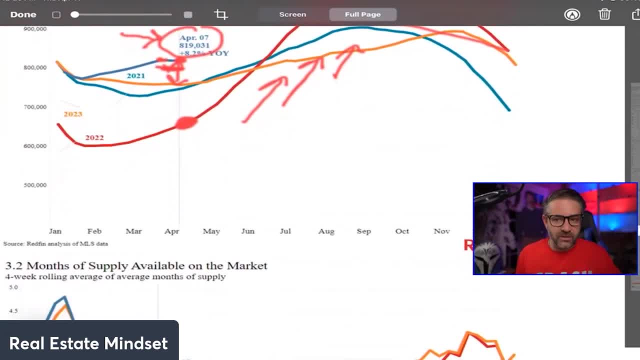 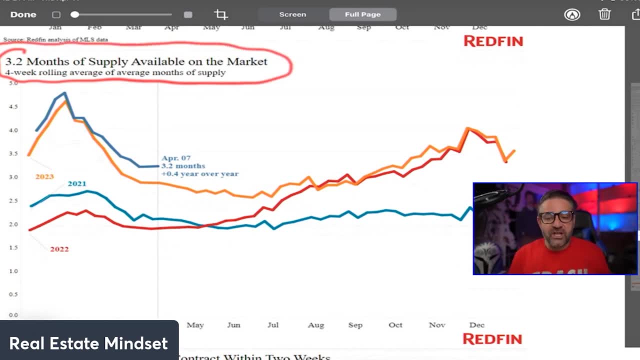 two weeks. it's been a plateau. that's not something that we want to look at now. but now look at months of supply. okay, months of supply. we're sitting at 3.2 months. everyone should know by now. we need about six months for the market to technically consider. it a buyer's market. i think we just need to sustain four to five months. just sustain that and we'll have our price discovery. but regardless, you guys, it has plateaued versus going down. this is good, but again we want it to go up. normally it's going to start going up right around july. 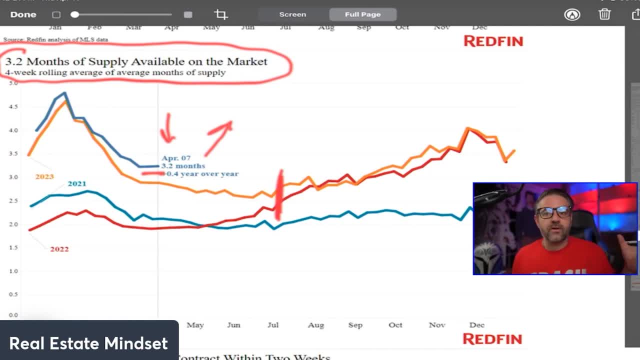 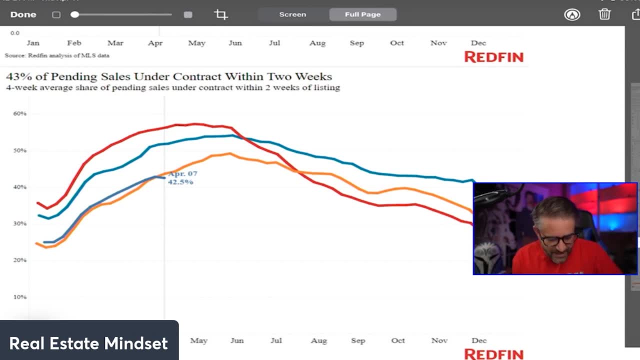 okay. so if it can go up before then that's a win for the housing market, in my opinion. this is also another data set where i see the housing market hit a brick wall. from the interest rates pending sales under contract in two weeks, so that's 43 of pending. 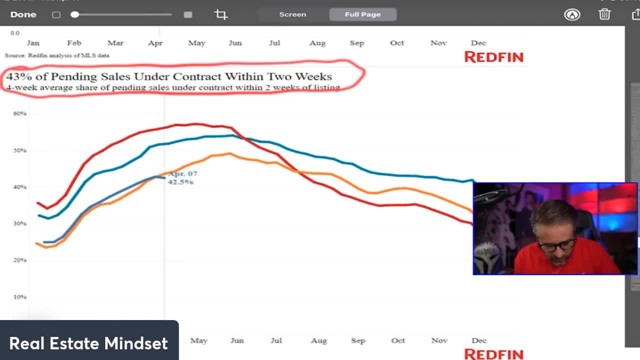 sales okay, which means pretty much demand. now again, look at the trajectory. it's like it hit a brick wall right. and normally again this time of year, normally we're in spring, right, normally it goes up. so the fact that it's going the opposite trajectory should tell us: this is good, these are. 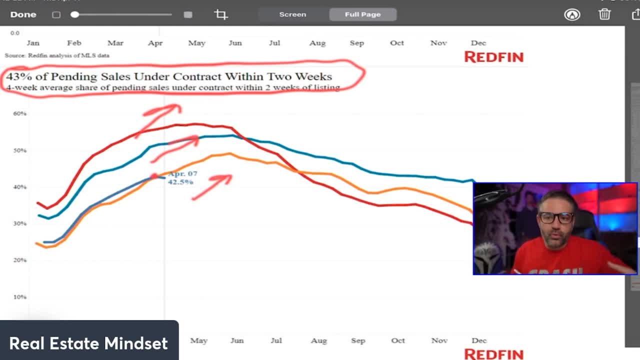 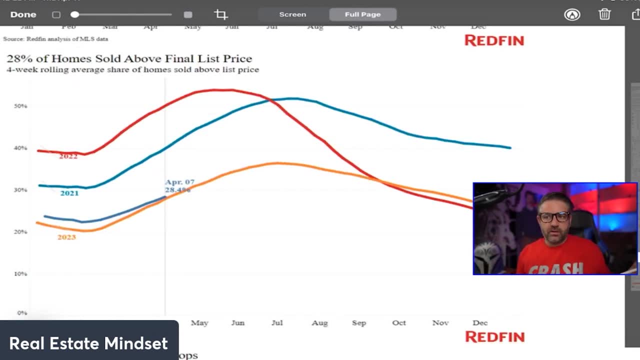 great things. we just need to hold right now. we need to hold where we're at, and these trends should do the opposite of normal seasonality. now, another lagging set of data, you guys: 28 of homes sold above final list price. um, you know, that's almost a four-year low. we still want this under 2023. we're. 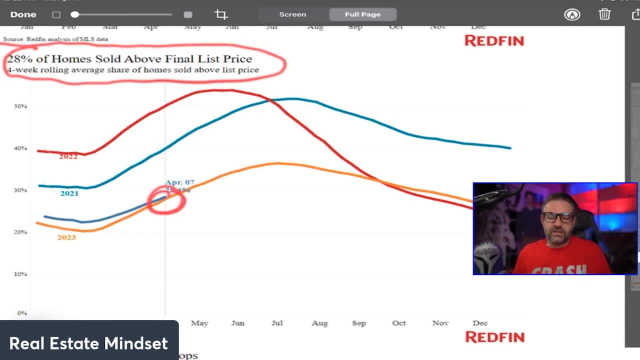 kind of right at it. you kind of can see that right there. but again, we want this down. we want things to be on the market for longer, because the longer they sit on the market generally, the more likely it is for sellers to start cutting the prices on their homes. 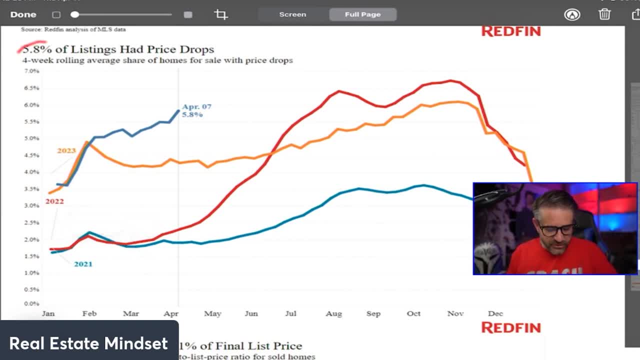 here's another great set of data, you guys, again opposite of normal seasonality, which the price is going up like. that doesn't make sense to me, because the price drops and price cuts are exploding- the opposite of normal seasonal trends, you guys, normally we don't have this type of price cuts. 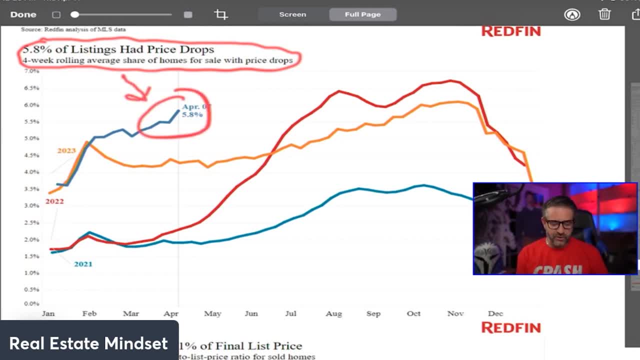 we're sitting way, way up here at 5.8 percent again. we don't usually have this type of price cuts until we're all the way over here, going into fall and winter. so thank god the interest rates are high right now in the seven percent because we can see that the price cuts are.